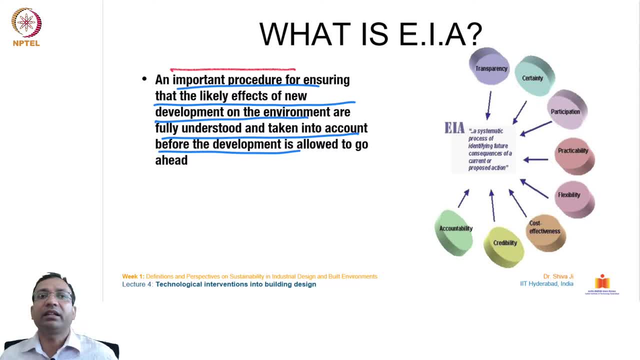 of like a, calculations and analysis of like a, any like a possible, actually plausible like a effect which an development process in a development activity is going to actually exert impact on the like a surrounding and overall ecosystem. So it takes care of like a with the help of. 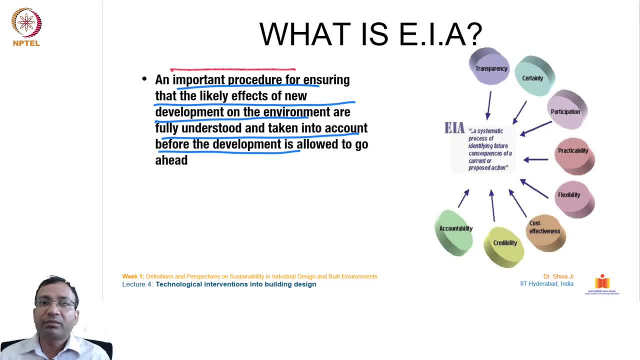 like a pre-M2, actually measures and calculations, So it is like a systematic process of identifying a future consequences of a current or proposed action. So that is what it actually does and that is actually main objective of like a conducting EIA. 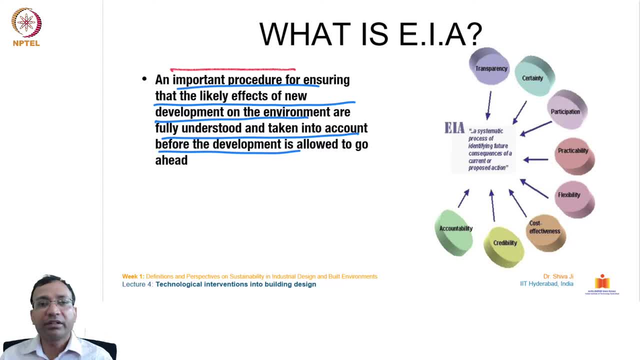 So it takes care of like a. it actually results into like a setting up, like a accountability. It establishes like a credibility. It checks like a cost effectiveness. It actually proposes like a flexible, like a ways to do things. It checks like the practicality, It checks like a participation. 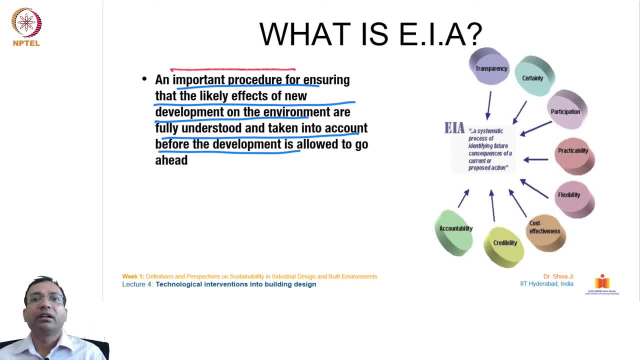 It involves actually people and different like stakeholders. It actually talks about like a certainty and then the other stuff which are going to like a, certainly like a happen and all that. So it talks about in a like a finite terms. It actually establishes a transparent, actually system of like a establishment, how, if we are going to undertake 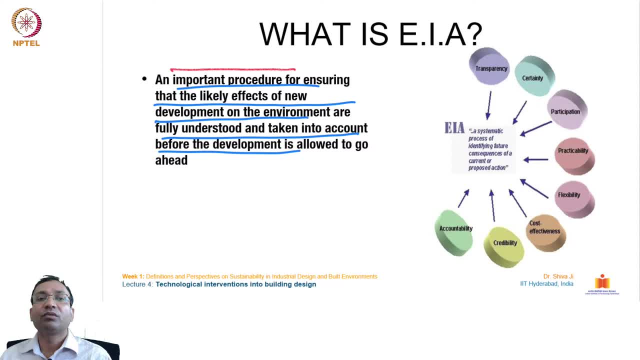 any like a development procedure, any like a developmental activity? So what are the plausible actually reactions or the repercussions which that place is going to fact face? So this EIA actually helps, like a pre-hand this analysis, like a pre-hand this analysis, to understand all of those things. 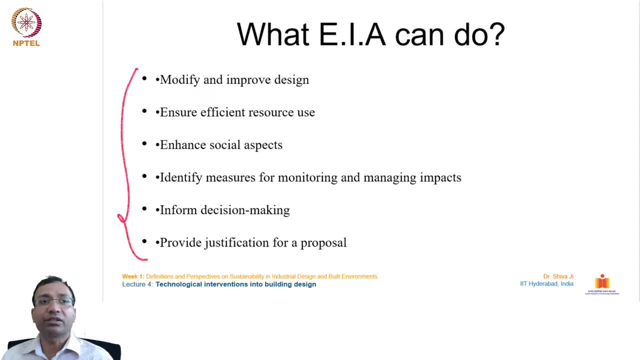 and it helps in taking up, like a an informed decision, So what an EIA can do, what this environmental impact assessments can do. So they actually are helpful in like a modifying and improving actually plan and the design of that, the developmental activity, what we are going to. 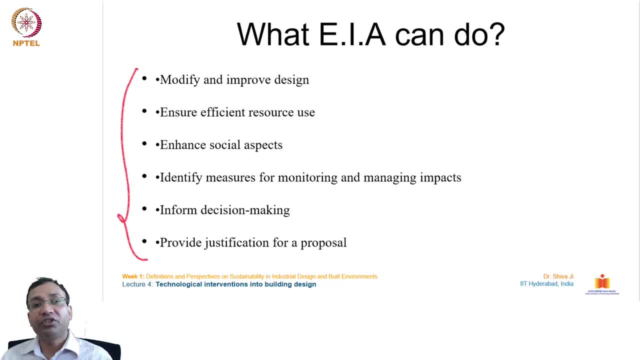 undertake. It helps in ensuring like a efficient resource uses. So it improves. it improves the actually usefulness, It improves the like a efficiency of like a resources, resource consumption. It enhances actually social aspects. It takes care of the like a society. It takes care of the like a. 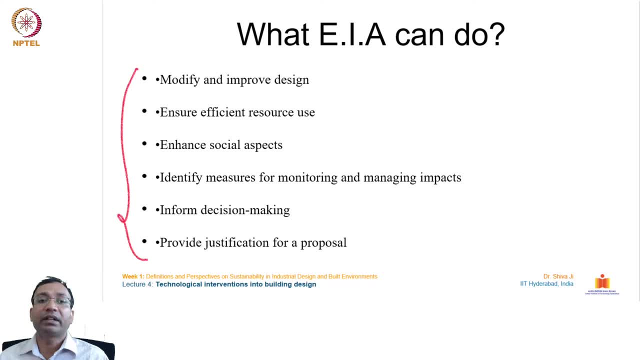 local community and the people and how this developmental activity is going to like affect them in several ways. It helps further in identifying measures for like monitoring and managing like impacts. So it helps in actually understanding. it helps in like a drawing, like a, you know numbers, in numbers you can understand, like how bad or how good is going to be like and what. 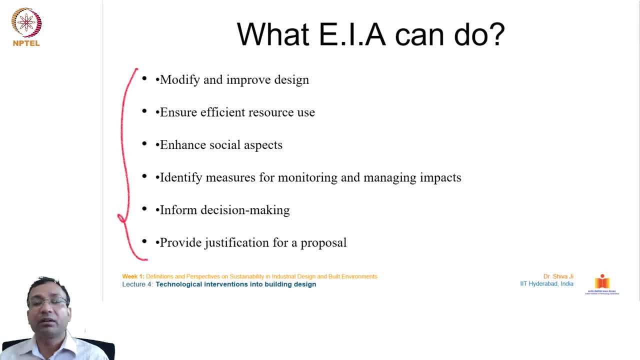 are the like, a different, like a kind of impacts, a plausible impacts in the like, a several, like a different domains, what we discussed in the previous slide. It helps actually in taking us like an informed decisions because once we are aware of like this kind of like effects are going, 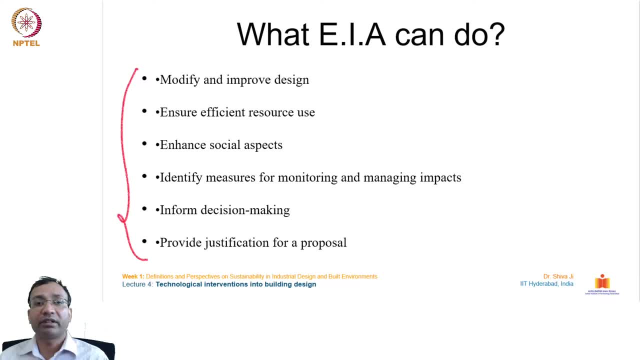 to like happen once the development process actually undertakes. then we can take some further, like a preemptive measures to minimize the impact of the environmental impact assessment, So we can actually analyze those impacts, for example, if there is a possibility that a certain kind of 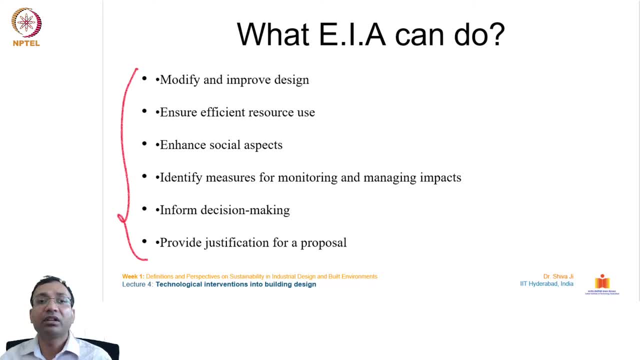 like a migration may be like a needed, some kind of like a relocation will be necessary for setting up like some, like a developmental activity. Then the rehabilitation actually processes can be actually taken care of to handle actually such situation and enable actually those people to establish somewhere else. So these are actually informed decision making. 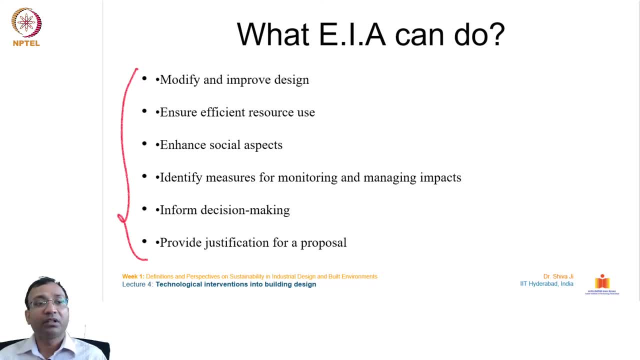 be actually taken care of with the help of like a EIA. the next comes like a providing, like a justification for a proposal. so if, if there is any like a, like a developmental activity which is proposed, so we can have actually some justification in terms of like a. what are the actually tentative? 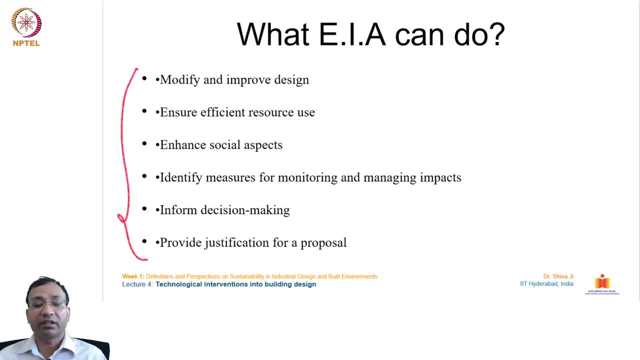 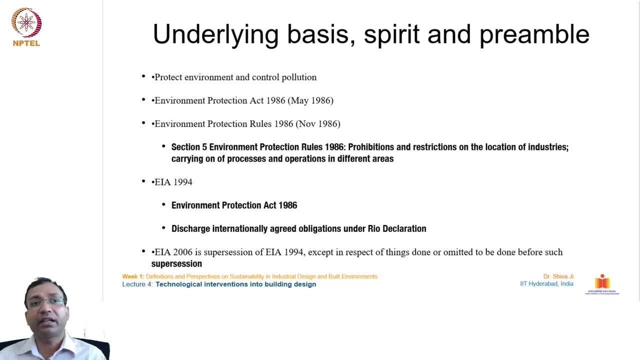 like advantages and disadvantages. the place is going to like a face next, if you see like a, it is evolving over like a period of time, like a. there are some. if you see some guidelines, some rules and regulations in place. there are some like acts established by the Honorable Parliament. 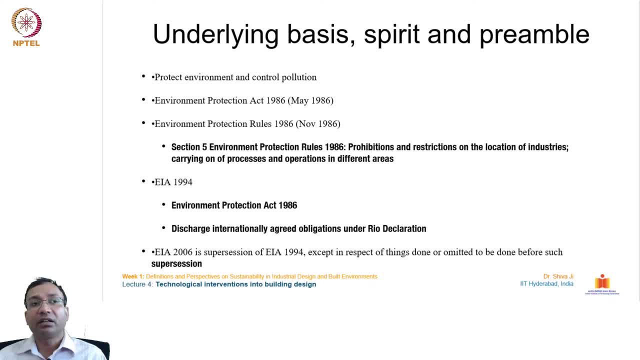 of India. so in that one, if you see like a, there are like a environmental protection and control, pollution control. actually rules and regulations are there, are, there are some are several bodies also, like a CPC, which is a central pollution control board. there is like a NGT, national green. 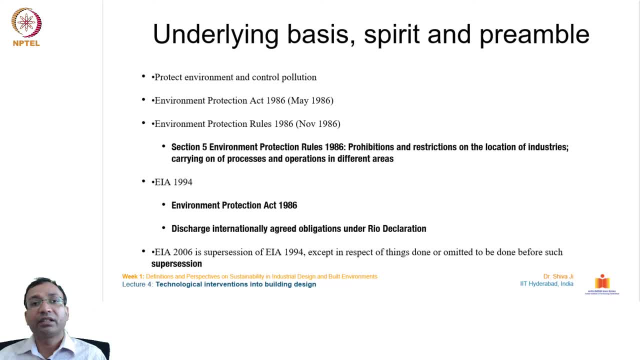 tribunal. so these are the actually. similarly, like, these are the several actually institutional. there are the, these are the several like a constitutional, actually bodies, organizations which actually take care of, like a such assessments, which actually take care of if there is something goes wrong with the as a. 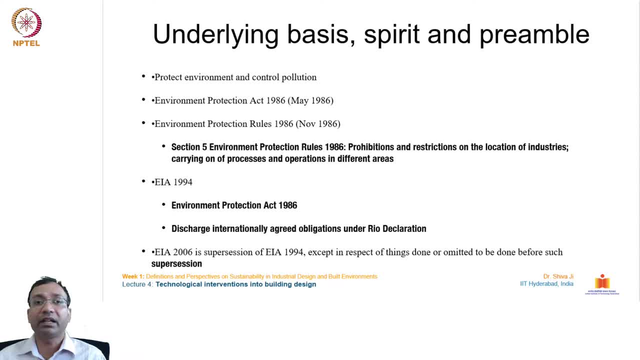 resultant of some development at developmental activity in any part of the India, so they actually come for the rescue of that place. they actually provide like a legal solutions. they provide actually with the corrective measures to cope up with the the repercussions which are like have happened due to like a such a like a bad developmental activities. so you can see there is like this: 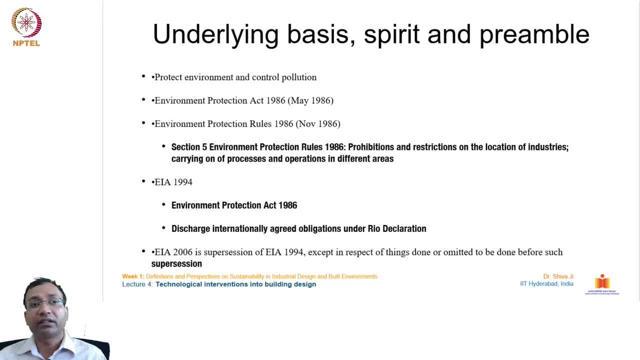 environmental protection at 1986. okay, there is like a another, like a set of like rules, environmental protection rules from like a 1986, and there is six and five which talks about like environmental protection rules 1986, prohibitions and restrictions on the location of like a industries carrying on of. 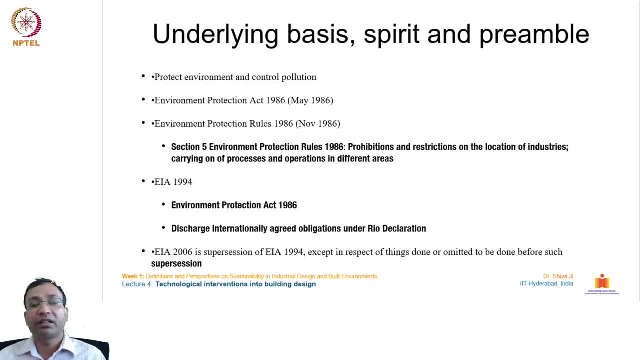 businesses and operations in different areas, and there is like a environmental assessment, uh like in 1994. this talks about uh discharge uh internationally agreed obligations under like a Rio declaration. so there are like a several uh international declarations also which our country, as a like a responsible country, has uh kept on actually agreeing to and it complies with those. 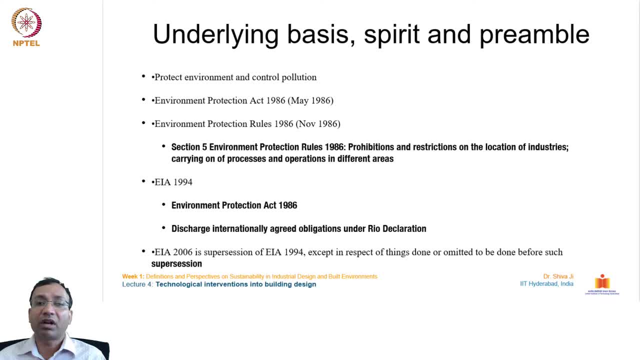 actually rules and regulations and mandatory like requirements which these actually protocols and declaration actually uh offer uh for the like a countries to adopt. so these, as we are all aware of all of these rules, regulations and uh declarations, they work in the like abettement of like uh. 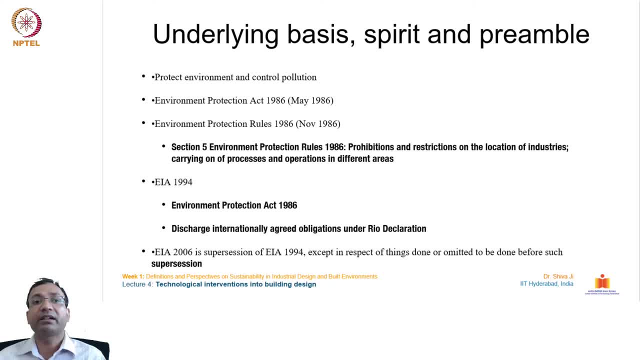 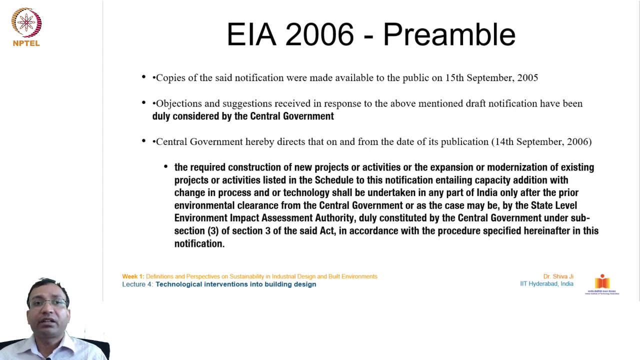 improving the atmosphere, improving the like ecological balance of this planet- not just one country including, like the entire planet- it helps in actually developing like sustainable models. so India also actually follows those declaration and has instituted several rules and regulation in compliance with those actually preambles. so if you see, like a eia, like 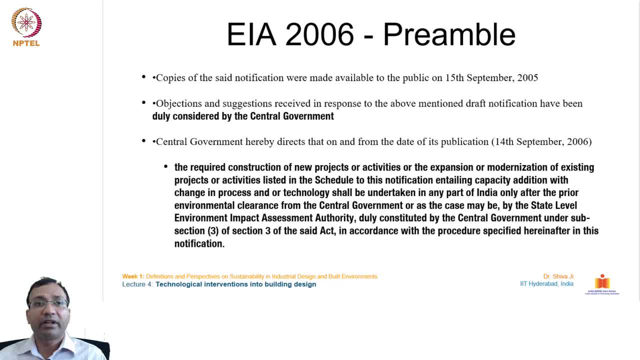 a 2006 preamble what it says. the copies of the said notification were made available to the public on 15th september, like a 2005. so and a standard practice in this actually sort of like activities is to involve like a stakeholders and the major stakeholder in any of like such. 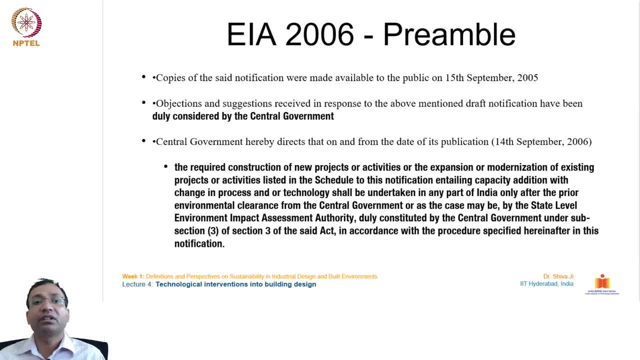 environmental activities is the public itself, because it's all like. all of these developmental activities are for the public and is for like a their benefit, and it is also supported by largely from the like a taxpayers money, from the like a public's money. so in a way or any like developmental 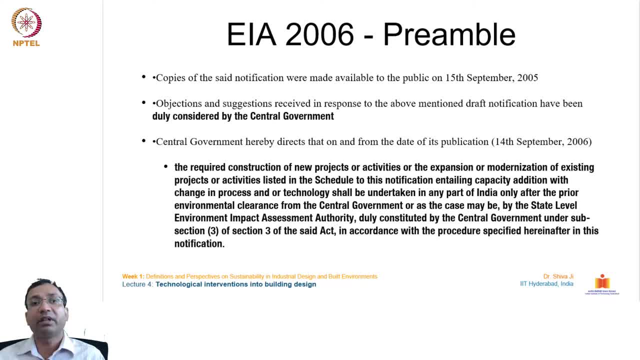 activity is responsible and is answerable to the public. so public must actually preview such like environmental assessment, like assessments, and they must actually approve of before going ahead with their developmental activities. so, as a like, an honor to that actually philosophy, this preamble was actually made available for the like, a viewing from the like a public on 15th. 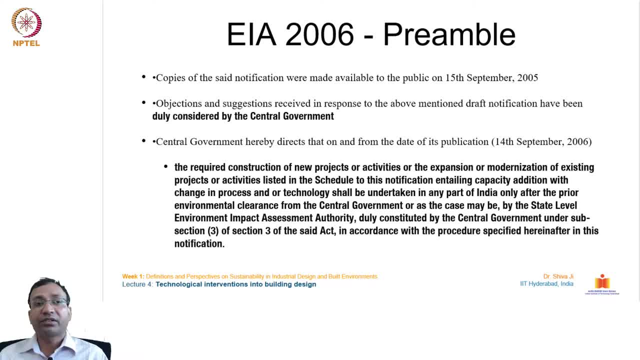 September 2005. so an objection and suggestions received in response to the like I ever mentioned, like a draft notification. so there were like a duly considered by the like a central government, and several like editings and corrections were actually carried out. so central government body hereby directs: 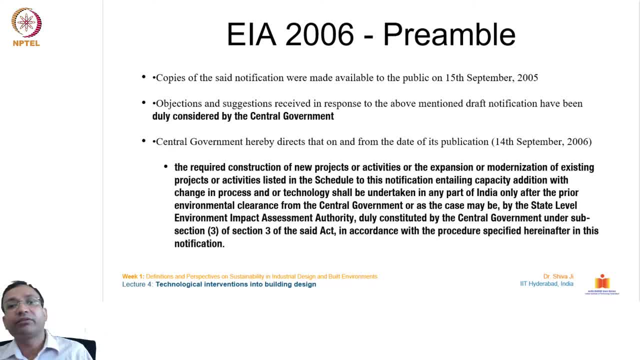 that on and from the date of its like a publication, that is, 14th of September 2006, okay, the required construction of new projects or activities or the expansion or modernization of existing projects or activities listed in the schedule to this notification in telling like a capacity addition with change in. 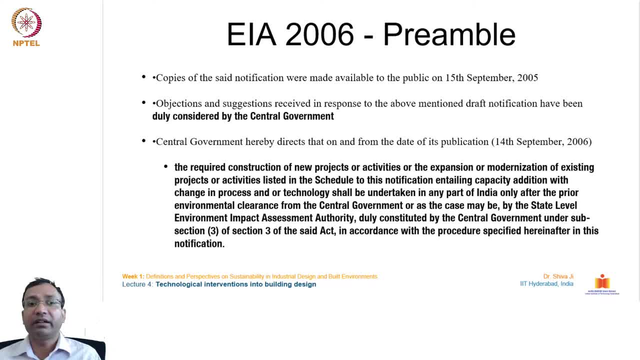 process or end or technology shall be like undertaken in any product India, only after the prior environmental clearance from the central government or, as the case may be, by the state level environmental impact assessment Authority duly constituted by the central government under subsection 3 of section 3 of the said Act, in accordance with the procedure, 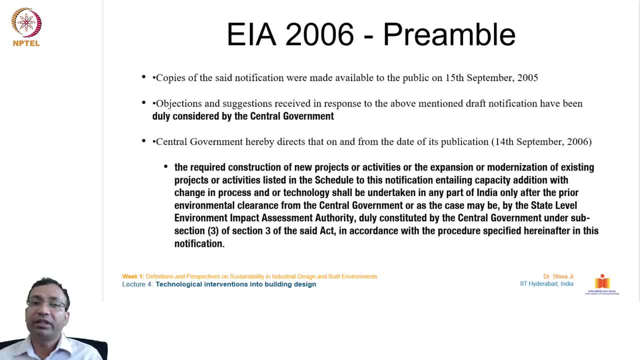 specified here and after in this notifications. so it clearly states over here- this preamble clearly actually makes its a point over here- any like a developmental activity which is proposed in any corner of India, in any state of India, she has to go undergo through this clearance of this environmental assessment Authority and get their 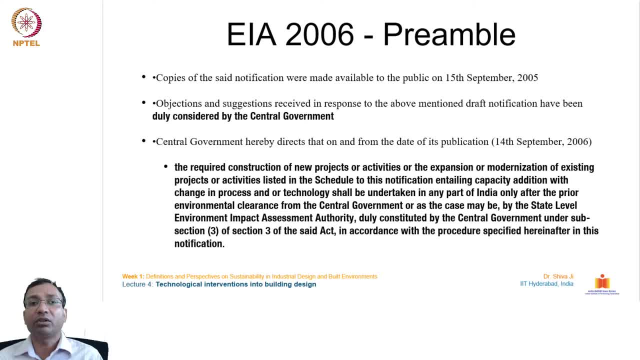 approval. only after obtaining that approval they can go ahead with the execution of that actually proposal and if need be, there may be some corrections and editings needed which must be actually carried out before actually going ahead with the development that activity. so if you see like as a summary of this EIA, like a process and rough, like roughly, like that, 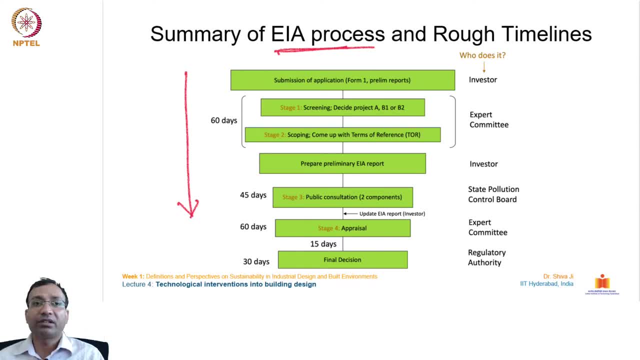 the timelines, if you see. so it starts from the submission of application, which is from number one, and it is submitted along with the like, a preliminary, like a report, such as like some assessment, some like a surveying and some like a data collection, okay, and etc. and then it goes further, like a screening, as a like. 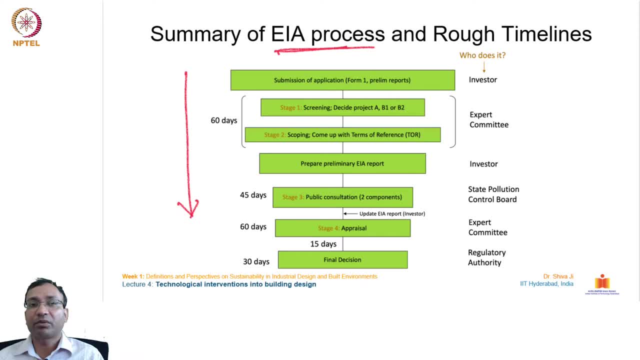 a stage one. so it decides so, like a based on the like, a project, like in different categories. and then it checks the like, a scoping income. it comes up with the like, a terms of, like a reference TOR. and then it goes further, like a preparing, like a preliminary EIA report, and after 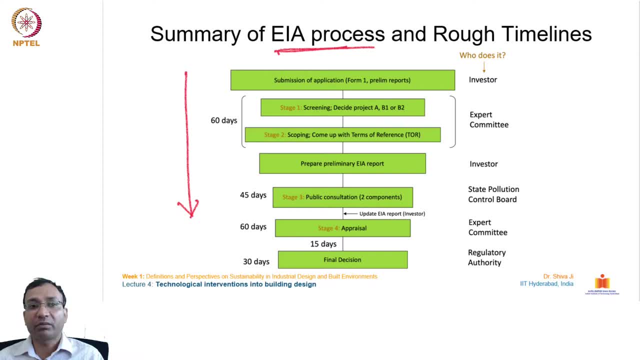 that a preliminary EIA report. it goes further, like a consultation from like a different stakeholders- public being the major stakeholder and a different other like researchers, NGOs and several other like an independent environmental protection agencies, etc. and after a consultation with the like a CPCB or state. 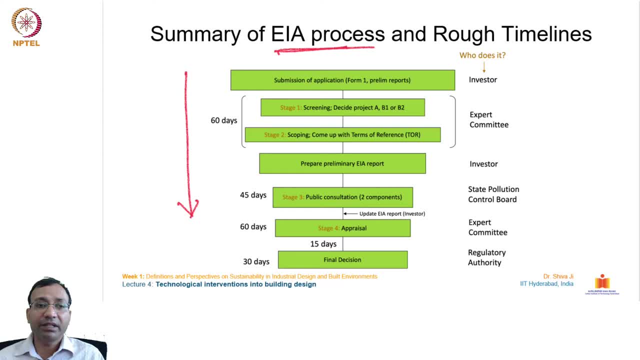 pollution control boards after consulting with the expert like a committees, then it goes for the like a appraisal. if there are any Corrections needed, that Corrections are actually advised to be carried out. further, the revised proposal goes for the final actually decision and here in after they actually go ahead with the their actually approval. so what are the? 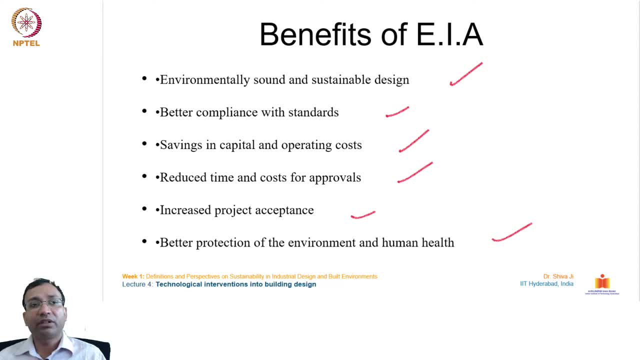 actually benefits of EIA. so it it helps actually in establishing like a sound and sustainable, like a environmental system. it helps in complying with the like a rules, laws and like a standards which are given by like a various agencies. it helps in like a saving the resource capital it's. it helps. 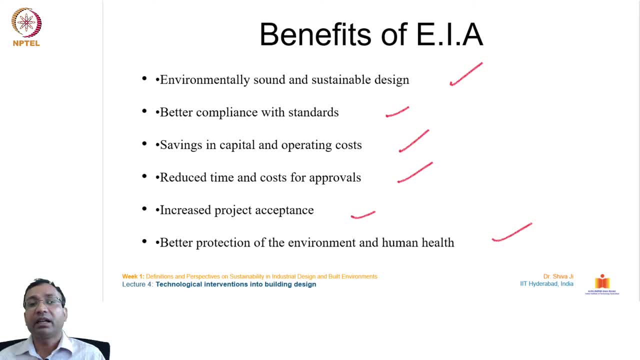 in saving the like a natural, like a resource capital of this planet and on the operating costs. it helps in reducing like a time and cost for the approval, because it's the one actually centralized, actually body for undertaking like any like such approval activities. it actually increases the project acceptance because, once it has gone through the rigorous process of this EIA, 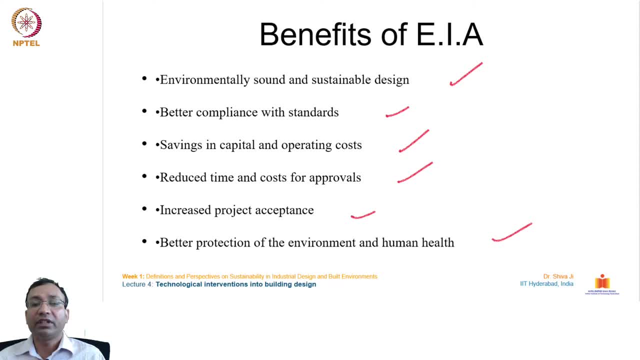 evaluation from the like authority, one can actually feel like a satisfied that yes, this project, once approved, can be actually not that bad and can be actually taken as a like an accepted level of like, a acceptance in the like a society and the community, and it offers like a better protection of the. 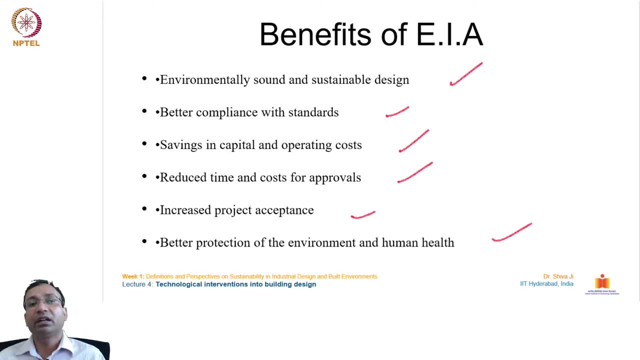 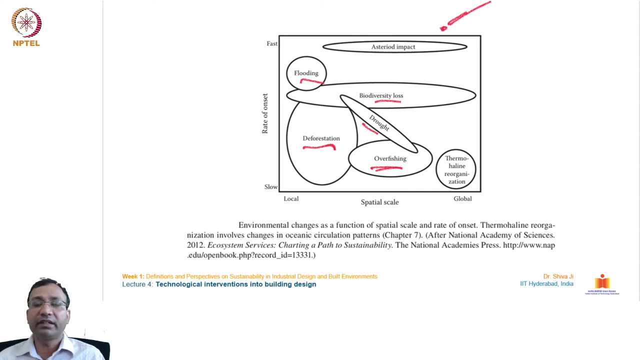 environment and the human health. so this is the actually overall objective of actually establishing like this is the environmental impact assessments so that sustainable, actually model of like a growth and development can be actually practiced in our like a real life. so in an overall sense, if you see what could cause the damage to our 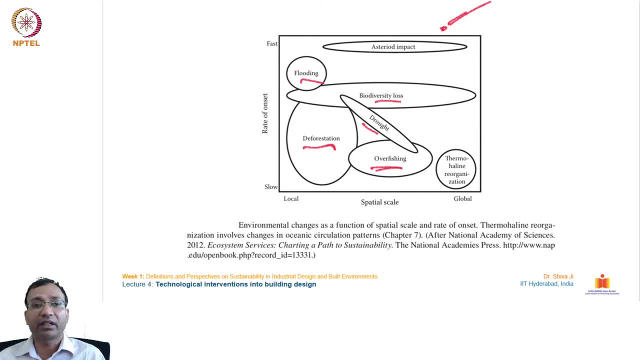 like a planet. so, on the excess x dimension, if you see it's like a on the spatial scale, whether it is local or global, or on the y scale. on the y dimension, if you see it is the, the rate of the onset, the, on the, at the rate of which, uh like how fast it can actually impact. so 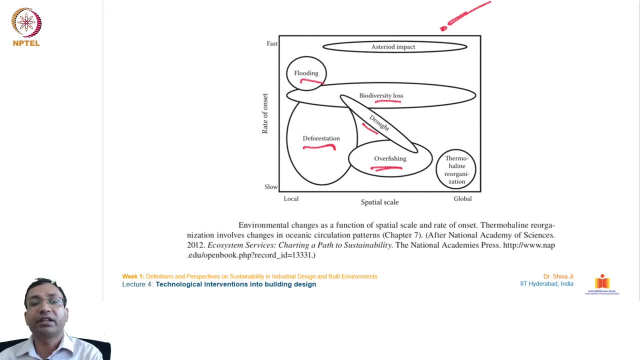 from slow to fast. so, for example- a weird example- actually asteroid impact is given at the top of it. so this has the actually potential to work from like a low local to the global level and it were it could actually, if it falls at any like unfortunate day- God forbid- it can actually. 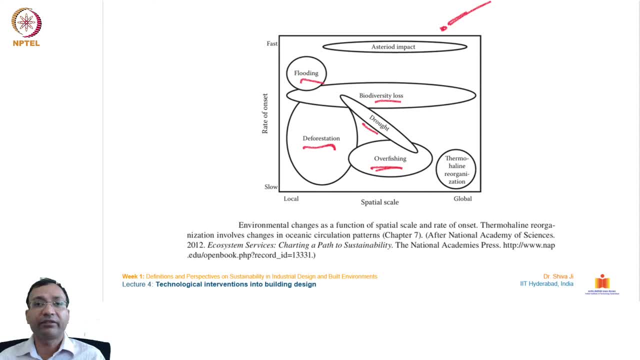 cause like extensive damage and it can happen actually at a very fast rates. so compared to that scale, if we see the other, uh not so noticeable, actually impacts. also, if we see which we, we do not actually see. uh, unless we experience it on our own, we do not actually. 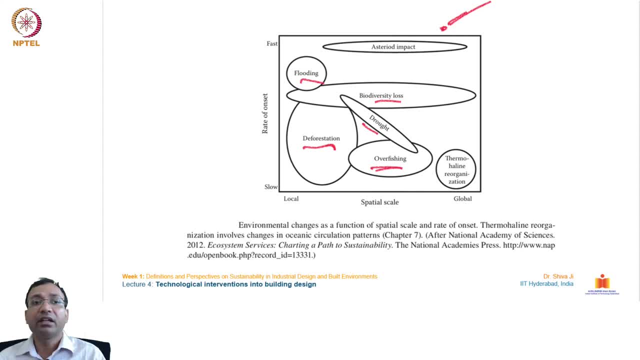 generally actually take care of these actually impacts such as like a flooding, such as like a deforestation, overfishing, you know, such as the, the loss of the like a biodiversity, like a components of the like of several species, you know. so these are also like such like indicators, which are 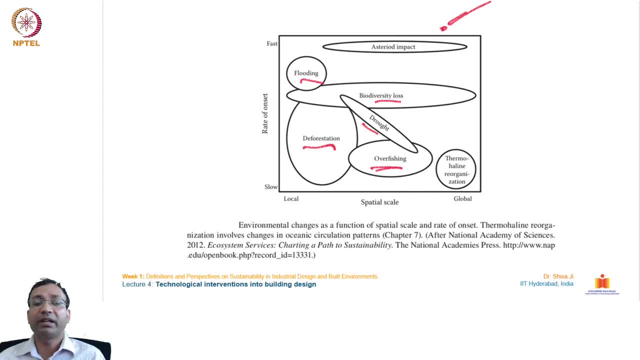 actually happening around us, which are actually destroying the planet bit by bit, every day, every year, every decade, and the other: Japan, Ged玉. the ecological balance of earth, biocapacity of of earth is in a serious, actually compromising situation right now and uh, how it can be actually uh, bring back to its normalcy. so this is the 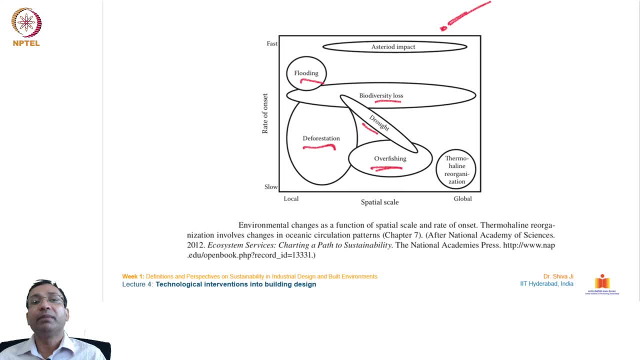 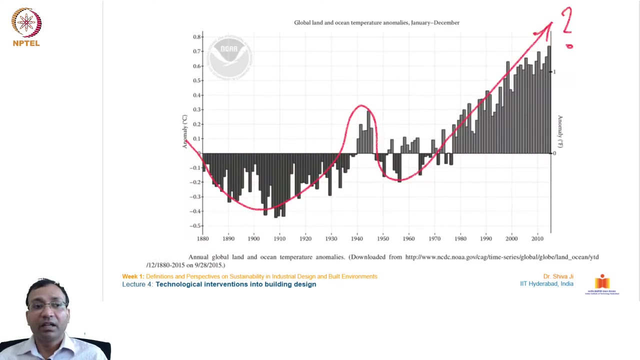 actually purpose of putting up this figure over here. the methods such as like a economic sustainability, the methods such as like a eia, they are there actually. they are framed for actually developing a sustainable model of actually growth and development and we must actually comply to those. uh, well, uh, such charts we have seen like a n number of times, like how the, like a annual, like 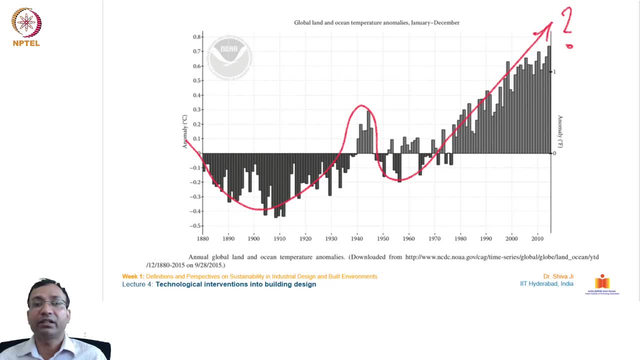 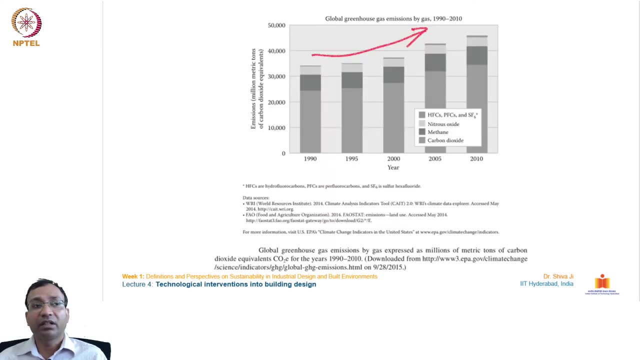 a temperature, uh how the overall, like a global warming is increasing like a on a like a yearly basis. well, it's uh increasing only so it's a major actually, uh, matter of like a concern and how, like a greenhouse, actually gas emissions are actually taking place. that is also a major actually. 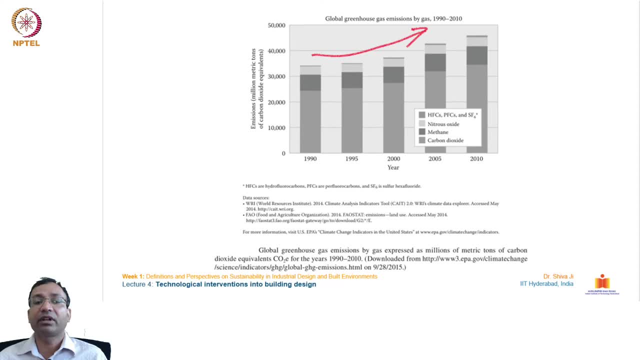 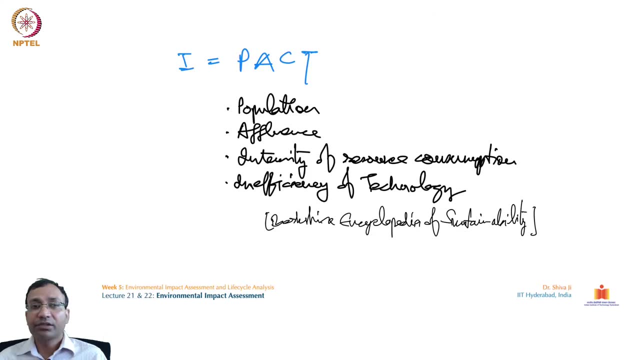 a concern which is the, actually a causing, actually factor for like a such like after effects, such as, like a overall, like a temperature increase and global warming, etc. so there is a and actually a model of like how to uh, calculate, actually impact. so with this, the analogy of this word itself, the researchers, they have actually given this concept. 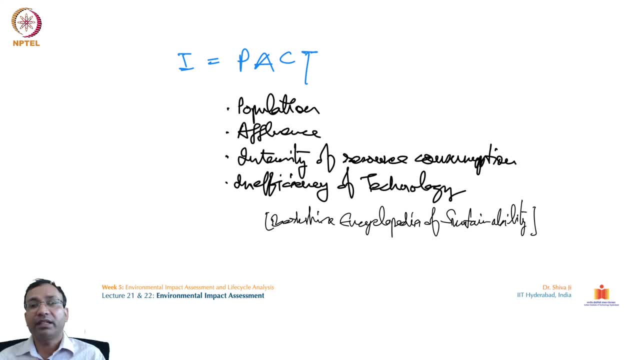 like i, is equal to p, a, c, t. so i is like the impact p is the like a population multiplied by affluence, multiplied by intensity of like a resource consumption, and that is again multiplied by inefficiency of the technology. so impact equals to a multiplication of all of these like a put together. so that is actually uh analogy, the 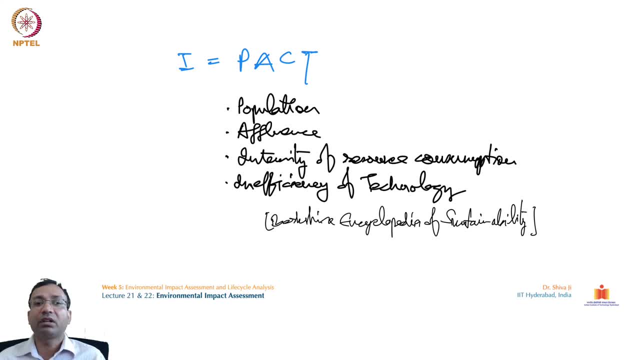 researcher has actually spoken about here and they have spoken about, uh, about the dematerialization also. so what is dematerialization? so like a um, going ahead with the actually reduction in the, like a consumption, going ahead with the uh, multiple uses of the resources, if it, if you. 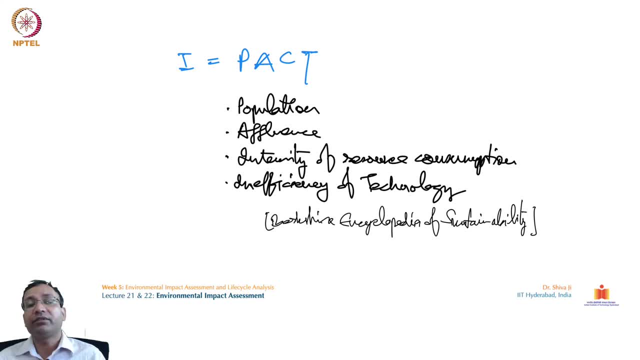 have to use that resource, then you go for like a multiple uses of it. if you have to go for the uses of that resources, then you go for the like a minimal, actually energy consuming a process or the way for like utilizing it or consuming it. so this is the actually uh, a concept of like the process. 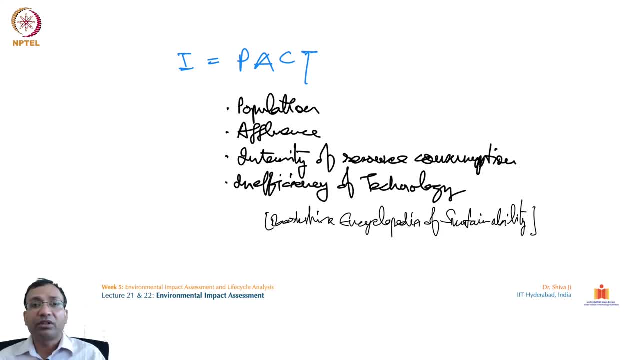 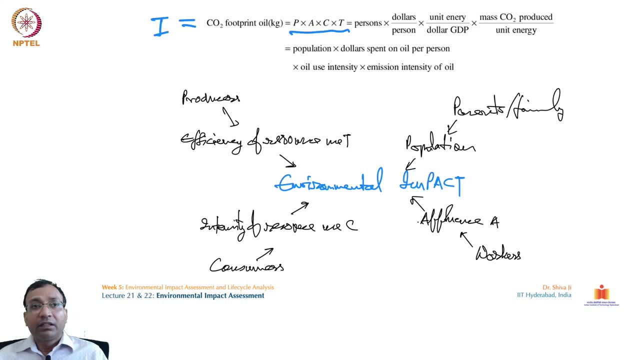 of like dematerialization, which could be actually helpful in reducing this overall like impact on this planet. yeah, so this is actually, uh, an illustrative actually diagram of this impact figure over here and here in this table you can see, like how the comparison of resource consumption levels for groups with low average and high ecological footprints. 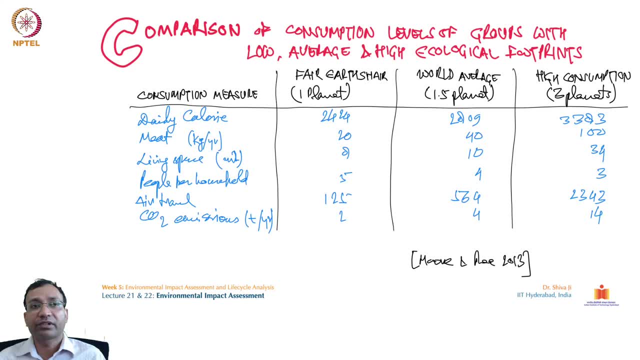 have actually taken place over the time. so the first column suggests about like a consumption measures, that is, like a daily calorie, like a supply, then like a meat consumption in kg per year, living space requirement in per square meter and then the people per household number of like a people, okay, and then home energy use. 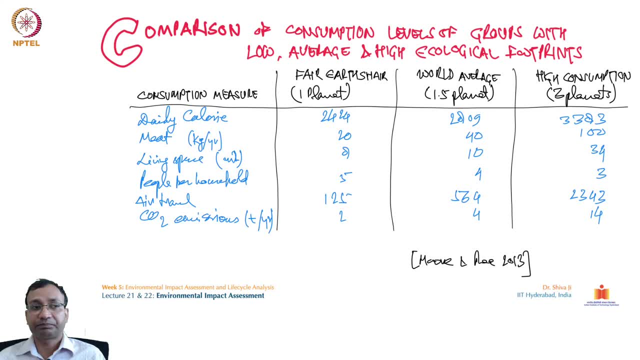 then motor vehicle travel kilometers per year, then air travels, then co2 emission a ton per year. so in this one, if you see that the fair earth share actually per combination talks about like a consuming, just the resources which can be supplied by like the one earth unit are the 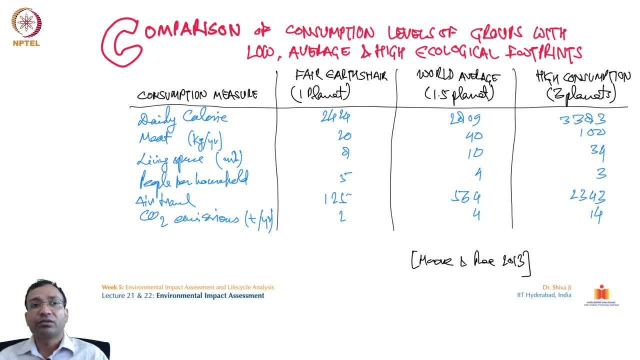 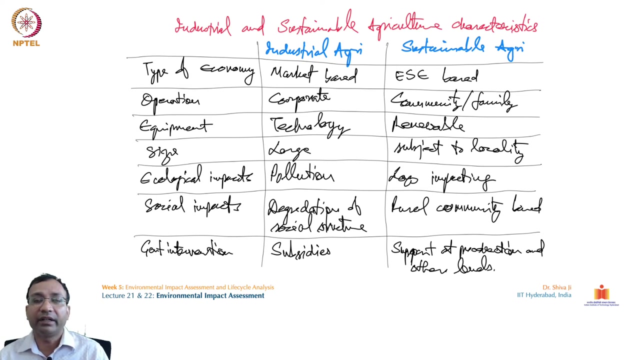 actually figures given over here like, for example, daily calorie supply. so the fair. actually earth is a different product from the natural resources, but you, we can sometimes see reasonable amount of electricity as the friendly energy were. um. this figure data, the uh, the consumption actually rate at which it has grown over the years. so on, this slide related to 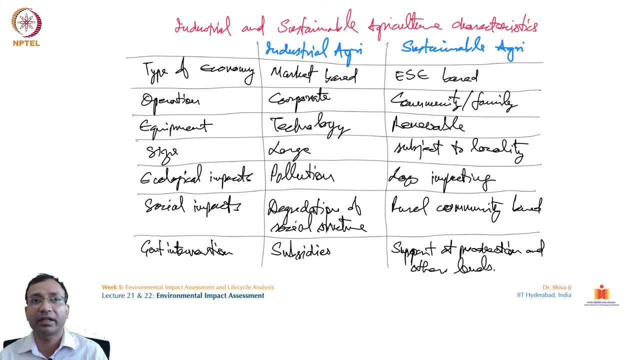 the previous one. it talks about like a characteristics of industrial and sustainable agriculture. so what are those actually uh uh factors, or what are those traits which we can associate from like a industrial, like agricultural system and like a sustainable agricultural systems? so well, till now, this uh uh in the post like a industrial era, so this industrialized way. 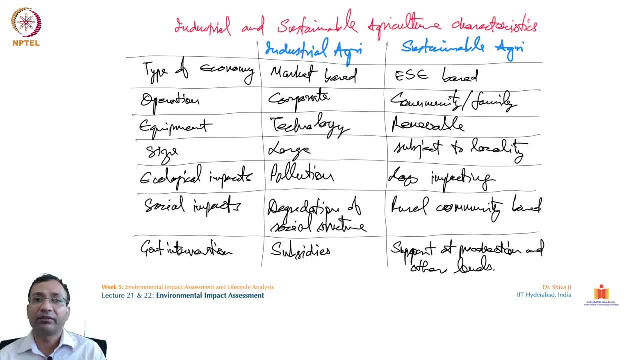 of actually agriculture has taken place and a lot of land, a lot of like a barren land, lot of like other like forms of land. they have been converted for like a crop cycles. they have been like a used with like a heavy amount of, like a fertilizers for the increased yield and several other like. 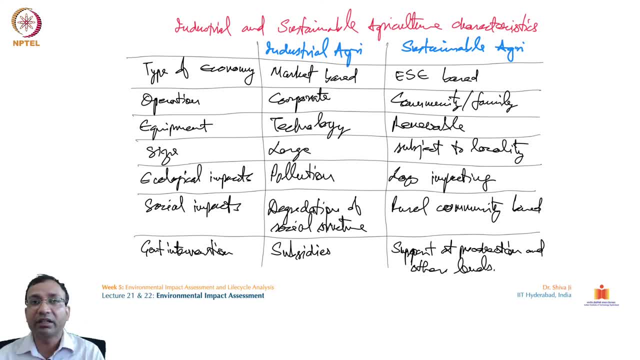 in the for the cattle's to in to boost like a deal to increasecieover here actually output for like a milk, milk and meat etc. they have been given with the several like hazardous, like a, like a medicinal, like a booster shots etc. to increase the overall like a amount of their like products. okay, so these are all the like industrial ways. 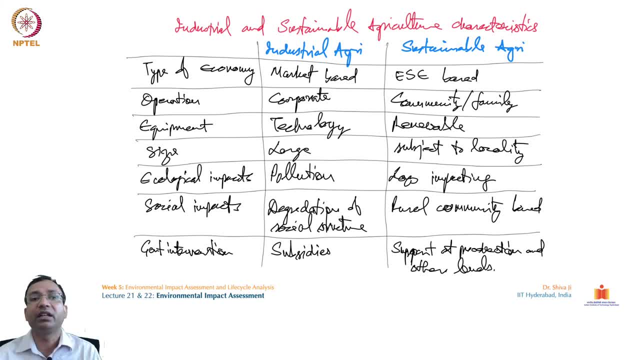 of actually agricultural system and what actually sustainability suggests is the like a sustainable agricultural practices. so we will see over here what are those actually poetic end? there are organization, there are muchos uh neg kinderen, disciplines, because they like land and its sort of. you know what are the existential level of agriculture? 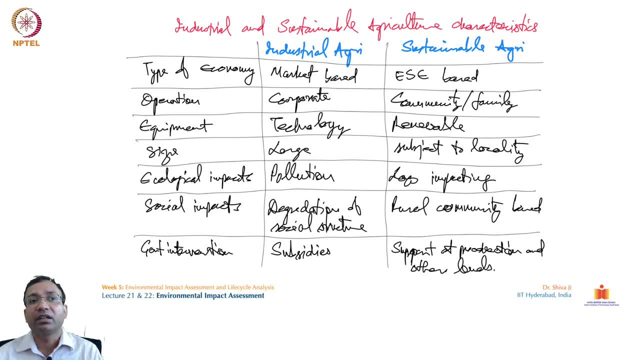 green and subscribe very easy if possible as well. so i legs, if you require manually, 왜 i sway? also points. so on the type of economy. if you see the again, industrial agriculture actually talks about a market based focused on, like a national and international markets. so the market and benefits. 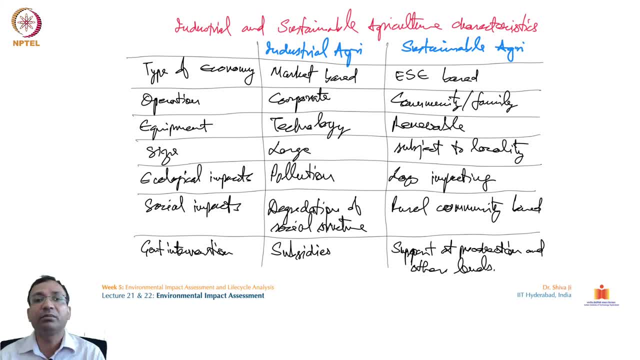 and actually creating like a economic wealth is the major actually criteria. but, on the other hand, in the sustainable agricultural system, the economically and ecologically efficient system, which is like oriented mostly on the local and regional markets, socially responsible, ecologically, like a friendly, so these are the actually keywords associated with the sustainable agricultural 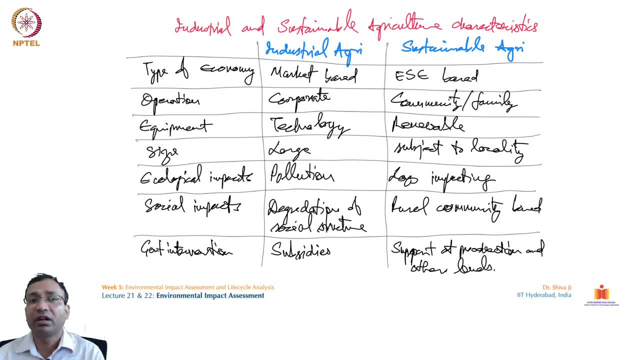 systems. so evidently it talks about actually a responsible way of actually using this agricultural, like a practices, in a responsible way of actually consuming a land for like a such, like a things it talks about and on the type of operation. if you see this, this actually operations are like. 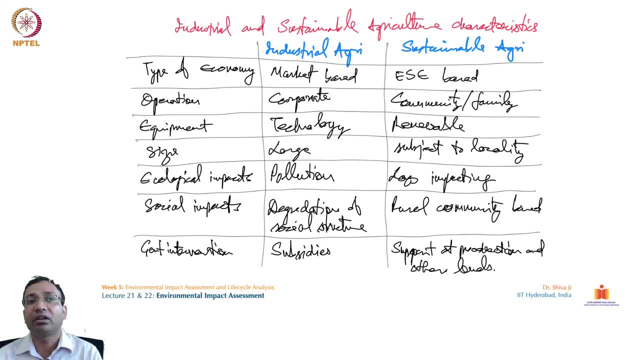 taken care of by management companies, corporate structure and on the other hand, on the sustainable agricultural system it promotes actually an independent, family oriented or community based, actually participation, where actually the social aspects, the social value systems are also actually taken care of, not just the monetary part. on the third, actually, 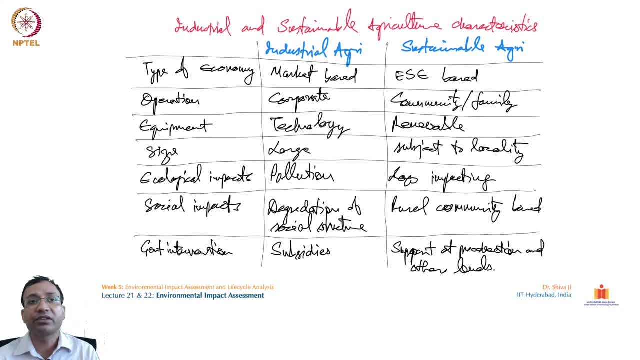 criteria if you see the size of the operation. so usually actually industrial agriculture happens at the very large scale, generally like a 500 hectares or even more, and on the other hand, like sustainable agriculture, actually takes place on a on a smaller level, like individuals, like a farmers, households based on their own, like 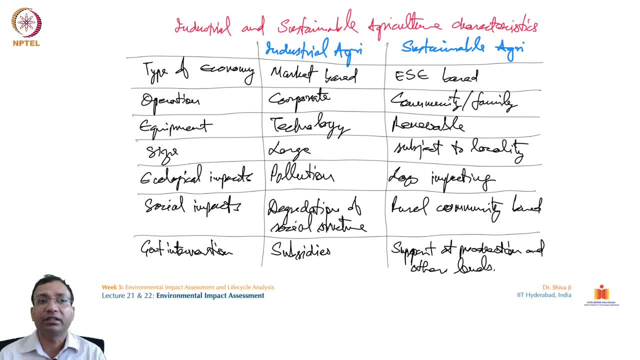 individual capacity they go for. actually these, the sizes of these operations actually take place. on the inputs front, if you see like a compared to like a, like a, what are the, the comparison? so in the industrial, actually agricultural- system, high levels of like industrial inputs, like a bio science. 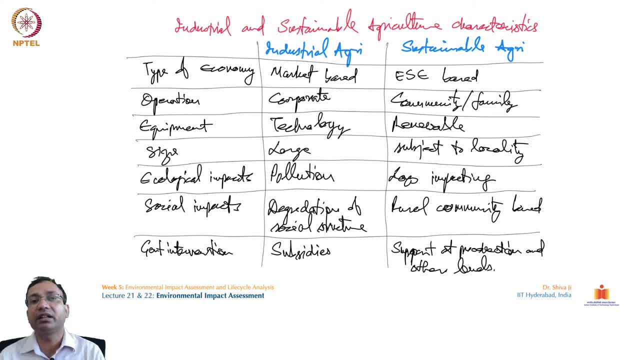 and nutrients in large quantities, fertilizer. so these are the chill kind of stuff- are really good. it is not just for the are given in the industrial agriculture. on the other hand, uh, in the second one, a few are like no industrial inputs are only the natural inputs, ecologically and integrated like a pest management. 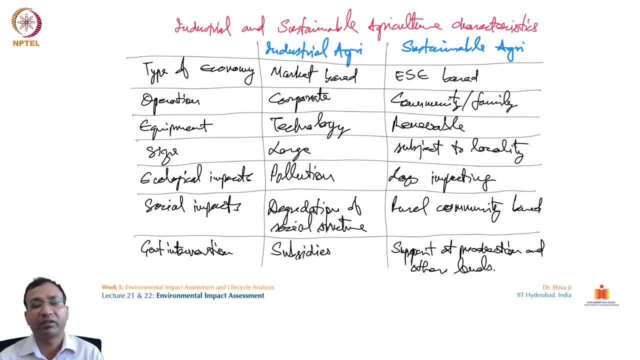 are given, which are very, very rooted to that place. there may be, like several types of, like a conventional knowledge is actually utilized in handling actually agriculture at the local level. so that is the philosophy which goes along with the culture of that place into the practice of the agriculture, also on the next front, if you see on the ecological like of impacts. so the major 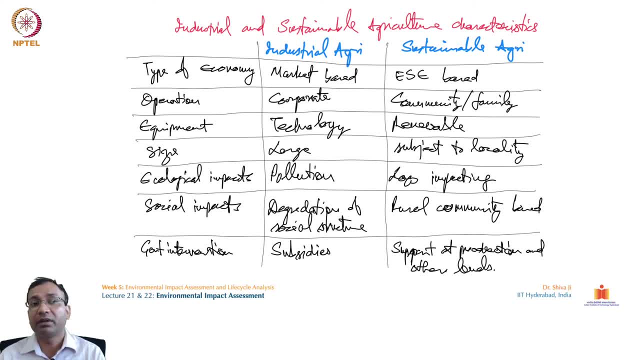 source of like a surface water, like a pollution, uh, it becomes like a major source for like a groundwater contamination also, because there is a huge amount of like a pesticides, insecticides and even fertilizers are actually utilized, so they end up actually uh poisoning our ecological balance of. 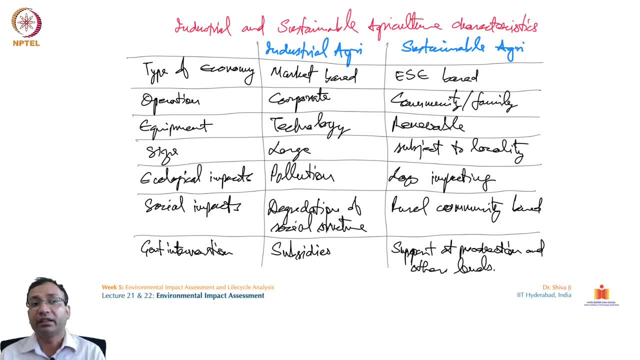 the water and the top layer of the soil. okay, they actually end up eliminating, actually, uh the habitat of the uh smaller like a micro, micro microorganisms and uh smaller like a small scale like microbes and other like insects which usually actually live in the like agricultural farms. on the other other hand, if you see this agrica sustainable agricultural system, uh it. 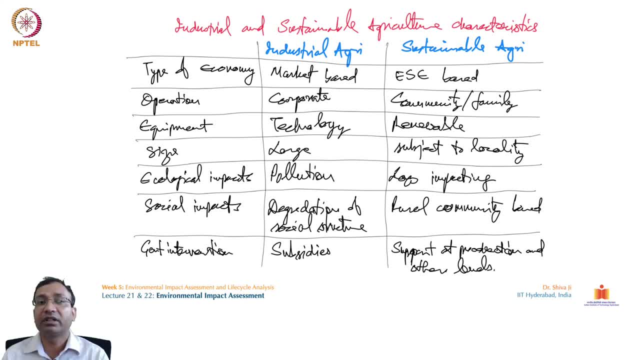 promotes actually low impact, uh and uh. it uses actually diversity of production, including like grains, fruits, vegetables, halves. so it uses actually it actually grows like a variety of agricultural produce, not just the one. not just it promotes the cash crop only, it promotes like other forms of like a crops also to have a actually a balance in terms of like. 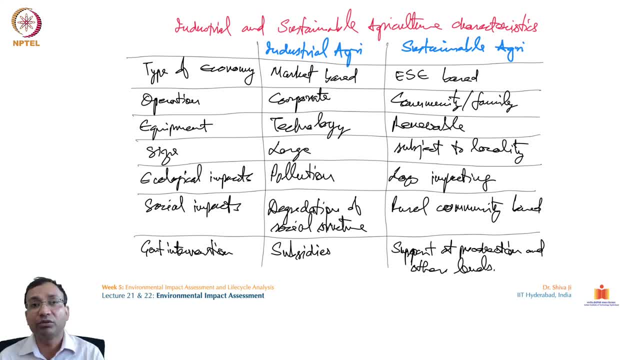 nutrients also because uh, we are all aware of like how the legumes actually uh help in adding like a nitrogen to the like uh top soil and how actually the other like a crop such as like a rice paddy, and uh these things and wheat they actually uh consume like a large. 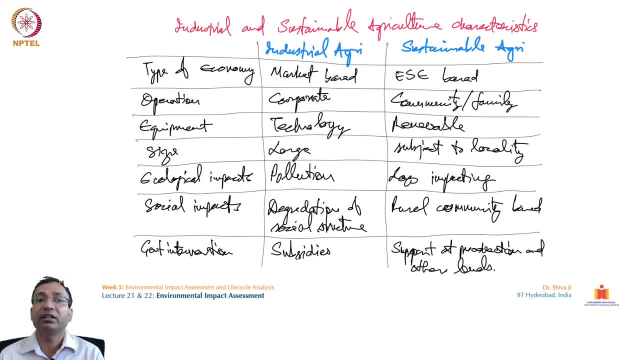 amount of like nutrient from the soil. so having actually uh, a circle of actually different like a crop cycles different actually grains and cereals, fruits and vegetables- it actually helps maintaining the nutritional value in the top soil. so sustainable agriculture actually promotes actually such practices. and on the next front, if you see, on the government intervention, there are a 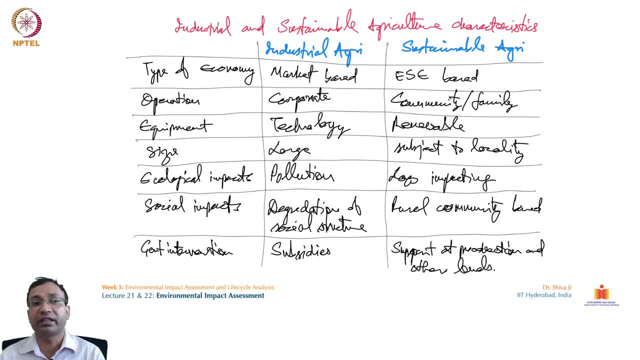 lot of like a subsidies and incentives available for like an industrial scale agricultural production on the sustainable agricultural system. if you see, like a government support for the production of non-market goods. it's supposed like a services, you know, ecological and social elimination of unsustainable input and production of subsidies. so it uh, the government helps in both the actually. 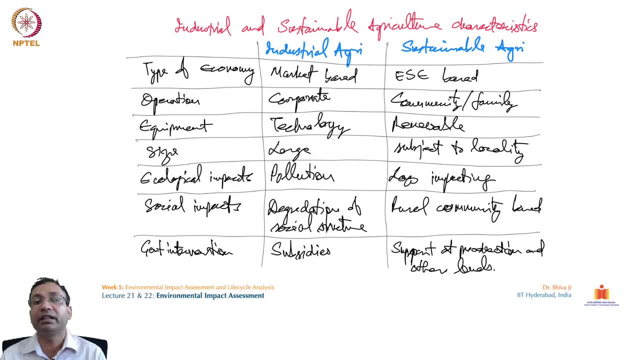 uh entities and, in the recent years, governments. like intervention has increased. the government support system has increased in the to support the small scale like a farming activities and farmers. uh, the last front actually talks about social. what are the social impacts of these two types of like agricultural practices? 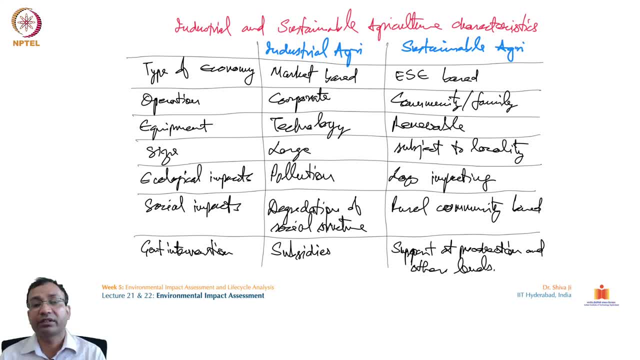 so here we see like uh the first one actually depopulates like rural communities uh, which leads to degradation of like a social infrastructure, uh the closer of like schools, collapse of like a housing market. so we have seen actually some uh like such impacts of like industrial level. 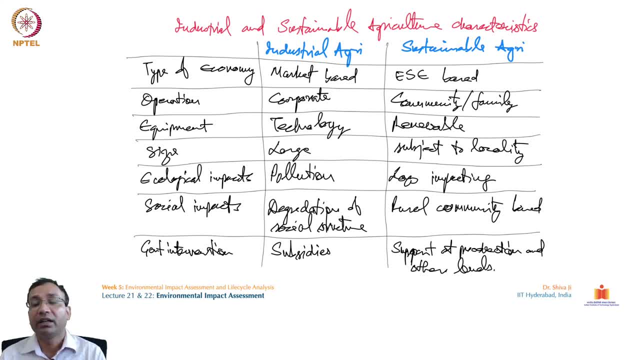 like agricultural practices because they uh employ uh a wide variety of like uh motorized and electric systems. in turn they employ a little like local uh labor force, man force uh to work on these farms and these like uh places. so in turn actually they end up a kind of- you know, a forced 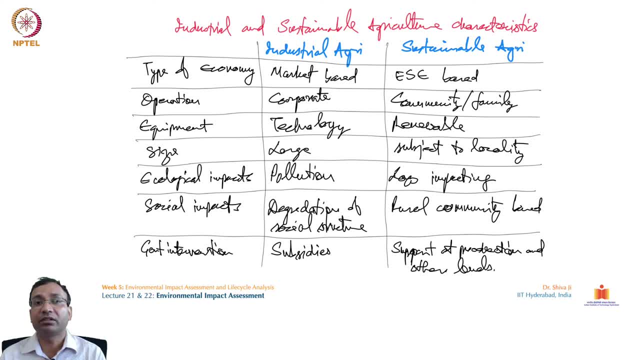 migration kind of a a phenomena, uh causing the people, causing the local people to vacate these places and move it to the other, like a greener areas. so these are actually some of the uh after, uh after effects in the like a social, actually uh area for the like uh industrial agriculture. 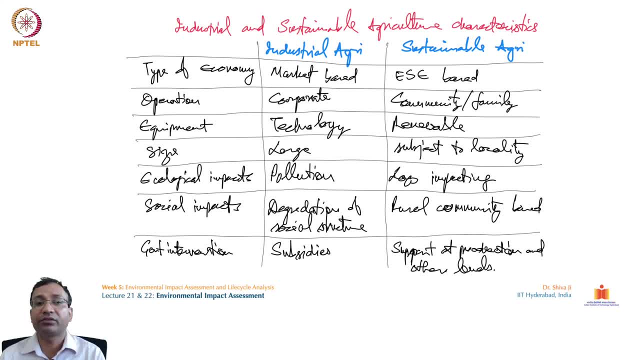 on the other hand, if we see, like, how the sustainable agriculture actually supports actually such activities, so which is actually beautiful to have actually a decentralized model of like economic, like growth and development processes, so it helps actually, uh, servicing like a local market, it provides like stability to the rural communities and societies, uh it. 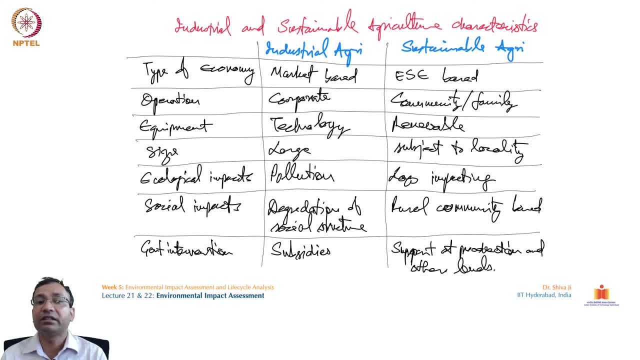 provides like economic, like a diversification, maintains cultural and landscape values, regional identity and traditions also. so we see there is a, there are actually n number of like a value systems which are also like a sustained and encouraged by actually sustainable agricultural system. so this is beneficial in like a multiple ways, like it helps actually the local market. it. 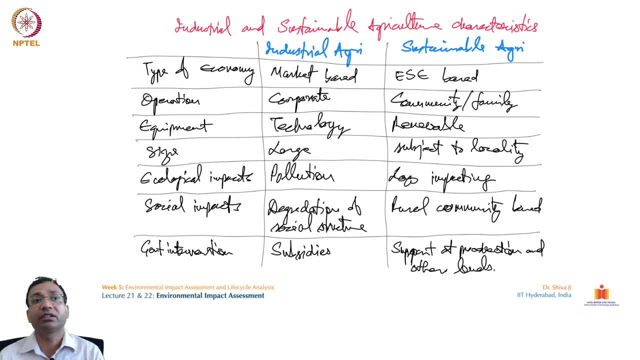 helps grow actually, the diversity of the product, because the industrial agriculture mainly focuses on, like a sustainable and sustainable developing and snacking of the products. so this is actually an an important, effective mechanism which viele of the different types of uh agricultural products that are available, like, for example, the really uh natural. 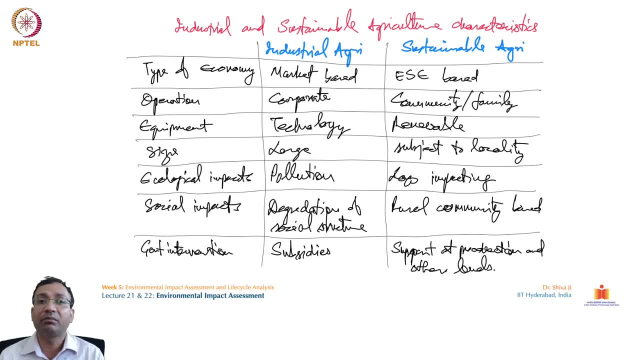 foods happen in the region. so if you are getting the traditional uh agricultural products, uh, there might be some uh like uh collage crops or the cash crops or the crops which are necessary uh for like the market or which are in a huge demand. but actually a sustainable agriculture actually promotes uh the local knowledge it promotes like. 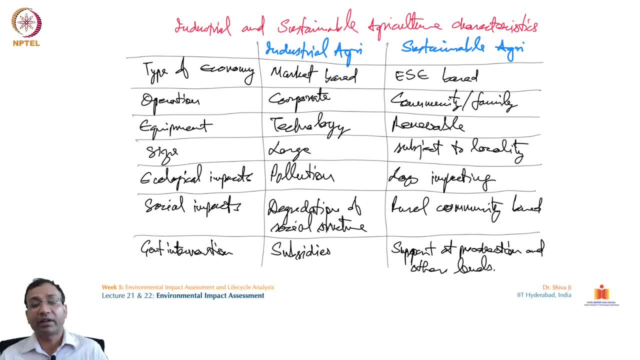 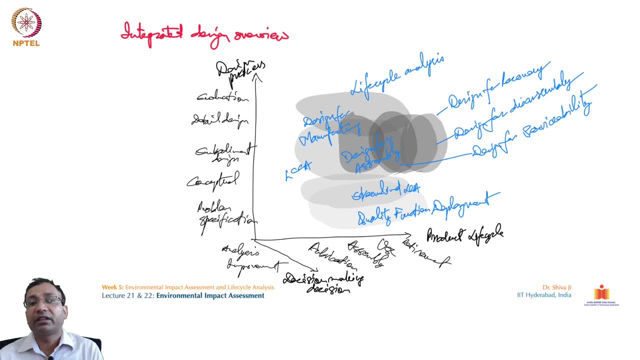 a local vernacular practices of the place and that is why it is a beneficial for the places. so, uh, what are the tools and techniques for like? if we see like a overall like, if you want to like a, have an, like a assessment, have a, like a impact, like environmental impact assessment, in like a? 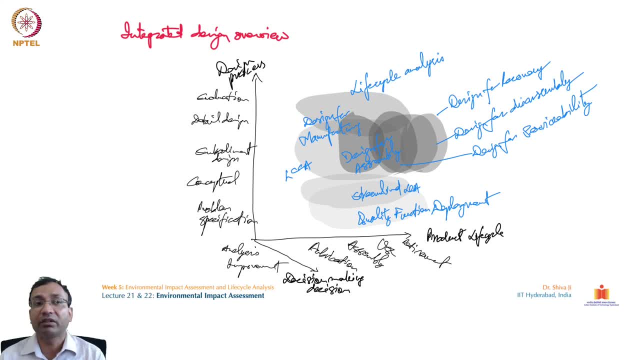 different scenarios. so if we see like this particular illustration over here, it talks about like a tools and techniques for like a integrated design, like a overview. so there are several types of like assessment methods and analysis, like a systems which are given over here in like xyz dimensions. so on the x dimension, uh, if you see it talks about like the product. 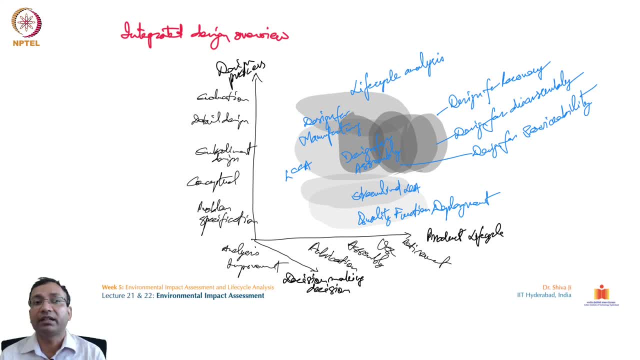 life cycle. so on that front, uh, it has like a scales of, like a fabrication, a scale of like assembly uses and the end of the life that is like a retirement or the disposal period on the y dimension, if you see, it talks about uh, analysis and improvement, you know. so it talks. 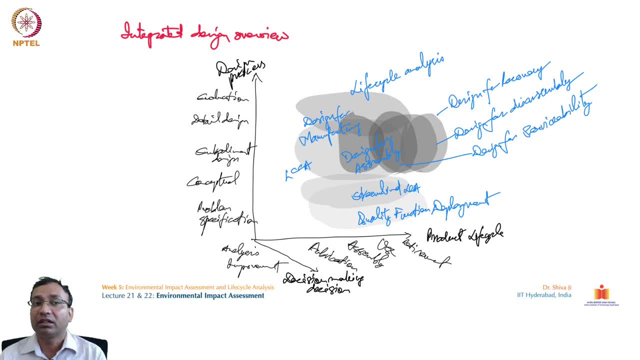 about majorly like a decision making capacity. uh uh, the the dimension of a part of this thing and on the z dimension, if you see it talks about like a design process. so what are the like a problem specification, what is the like a conceptual design? what is like a embodiment like design? what is like 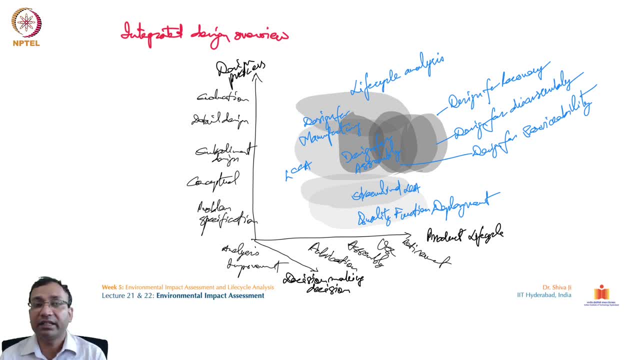 a design, detailing and what is like evaluation, etc. so at these, like xyz actually coordinates the methods such as like a dfd- design for like a disassembly, and dfs, design for like a serviceability. dfr- like designed for the recovery. dfa, that is designed for like assembly, dfm, designed for like a. 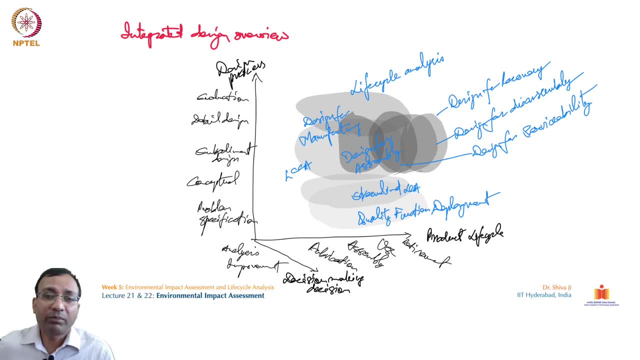 manufacturing. q. fd like a quality function deployment. lca that is like a lifecycle uh assessment, uh. slca that is like a streamlined, like a lca and lcca that is like a life cycle cost analysis. so these are the actually different assessment methods and different actually approaches for evaluation and even like a planning, these, these 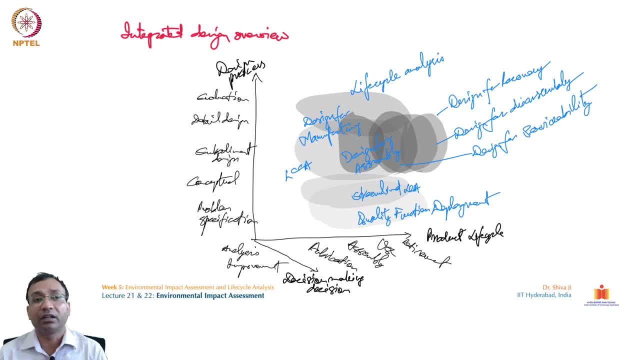 are actually placed to suit, which actually suit these actually particular actually combinations. so this actually gives us a comprehensive idea which kind of tool or which kind of actually approach would be actually working more suitably in which kind of like a scenario. so this is very, very far actually beneficial for our understanding. so we as a like a designer and architect and 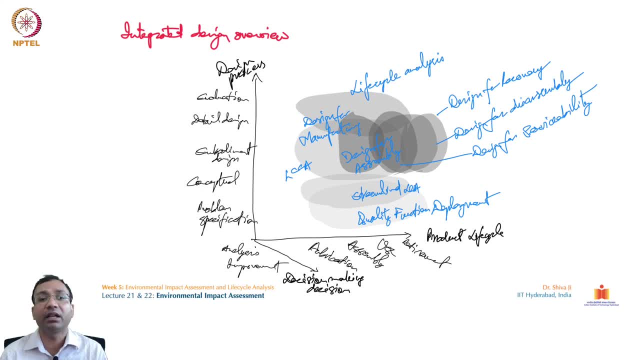 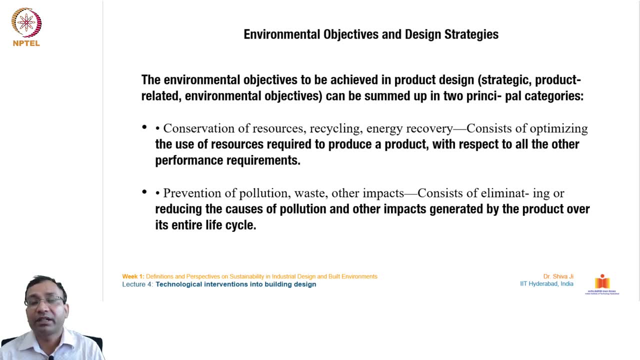 engineers can actually apply these tools in the appropriate, actually, situations. so, lastly, what are the like a environmental objectives and design strategies I would like to talk about over here? is the like a deliver moment, environmental objectives to be achieved in the like a product design? uh, with the like a strategy and product related, or